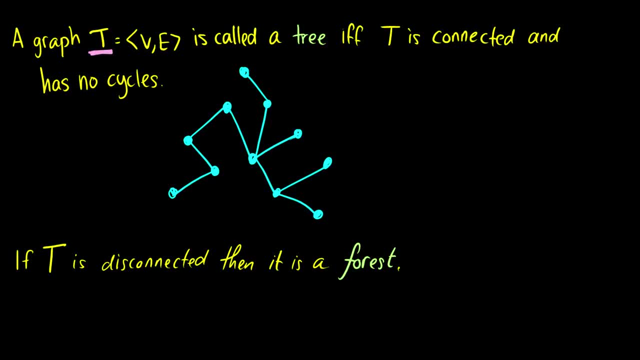 to denote trees. So if I use T, I'm talking about a tree. if I use G, I'm probably talking about any graph. So that is the definition of a tree. If you have a graph that is not completely connected but still abides by not having any cycles, then we call it a forest because essentially, this graph 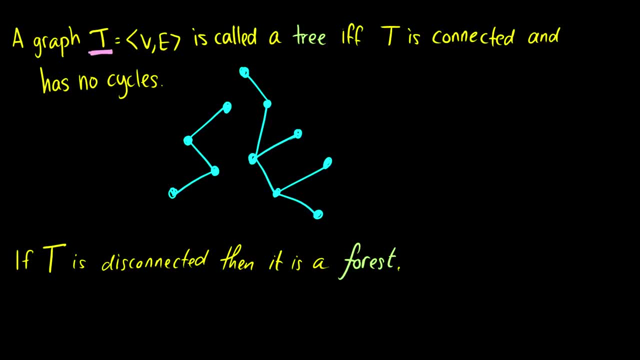 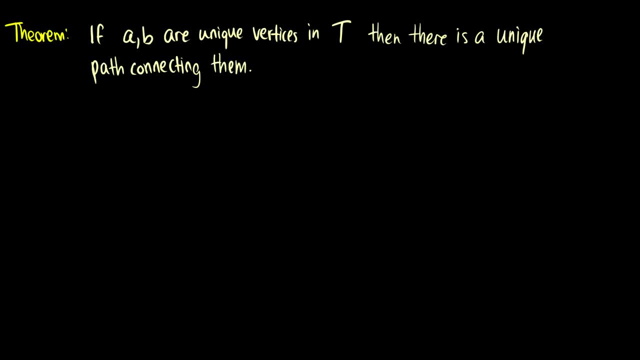 a tree. So let's start with a tree. So let's start with a tree. So if we have two vertices in a tree, then there's going to be a unique path connecting them. So I'll draw a very basic tree here. We'll. 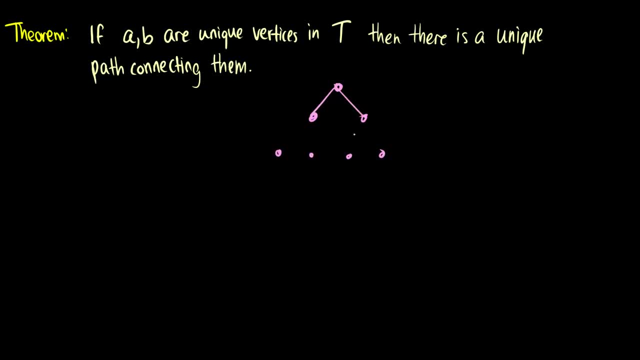 do a binary tree. So a binary tree always splits into two. So we'll do one more layer on some of these, Okay, and then one more here, And we'll pick a vertex A down here and we'll pick a random vertex B And we're seeing that we have two vertices in a tree. So we're seeing that we have two vertices. 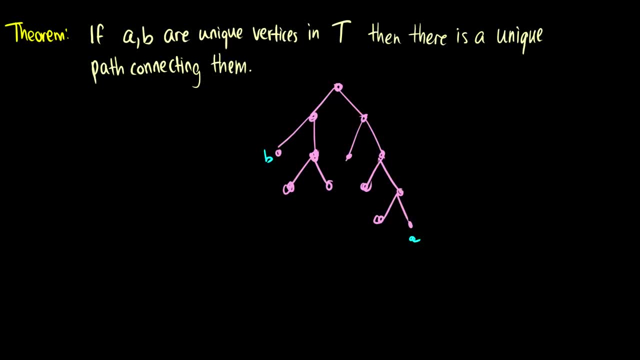 in a tree. So we're seeing that there's exactly one path to get from A to B. So remember, a path is a sequence of vertices such that none of them repeat. So we can see here that we go up, up, up. 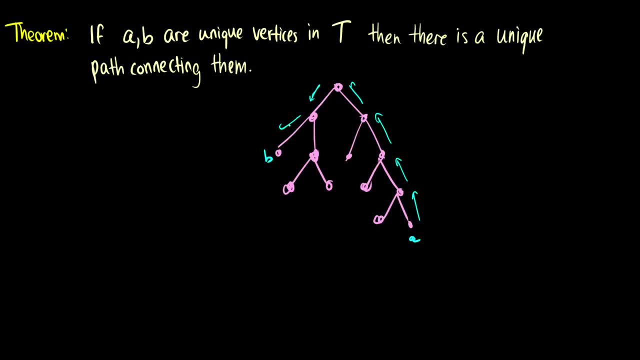 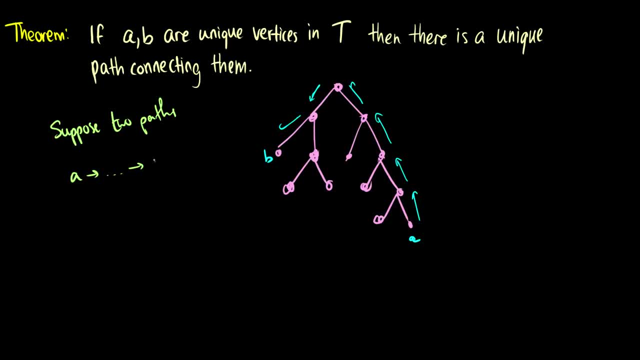 have two paths. So we have two paths. So we have A goes somewhere to B, and then we have A goes somewhere to B, But in here there's either one vertex or two vertices that are different. So we can say: this goes to some sequence X and this goes to some sequence Y. Well, what that means, 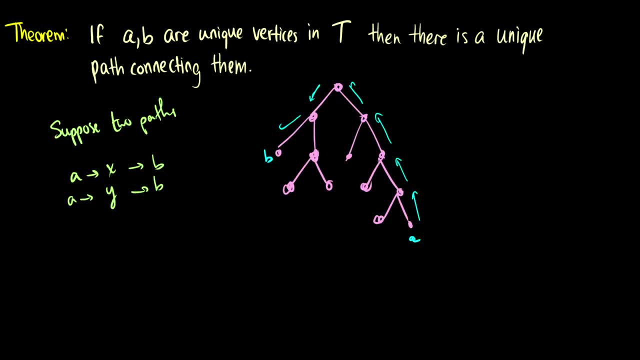 is that there has to be some loop somewhere, because we can either only go up or down. a tree can never revisit. So what this says is that there'd have to be a loop and therefore we have a contradiction with the definition. You could write a more detailed proof, but this is one of. 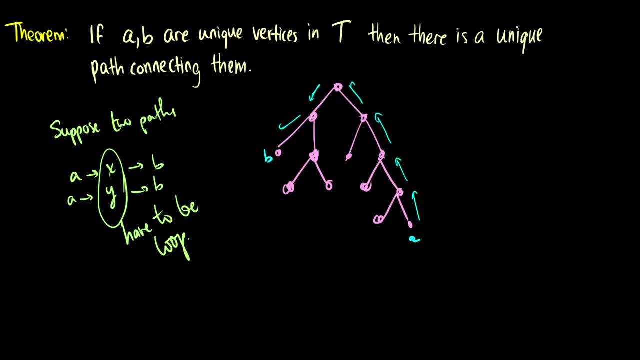 those properties. that is really, I'd say, obvious, and on an exam I don't think they'd ever make you prove this. So that is that question. The intuition is there. So let's move on to something that you probably would have to prove on an exam, and that is the property that in every tree, the number of 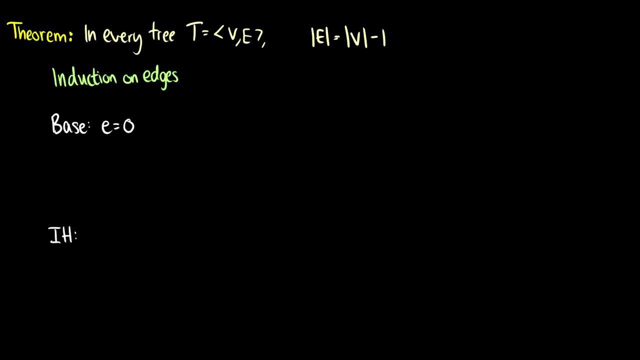 edges is equal to the number of vertices minus one. So let's do some intuition first. again, If I have three nodes in a tree, there's no loops and they all have to be connected. So I can connect it like this and like this: Two edges, three vertices, So three minus one is two. 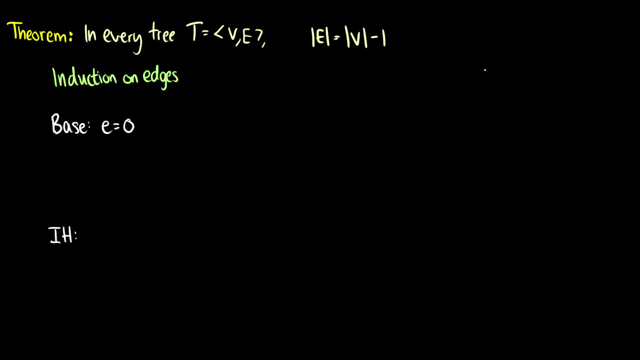 It holds. So to prove this, we'll do an induction on edges. So here we go. The base case e is equal to zero, So there's no edges. What does that mean? That means that there is one vertex. So this is: 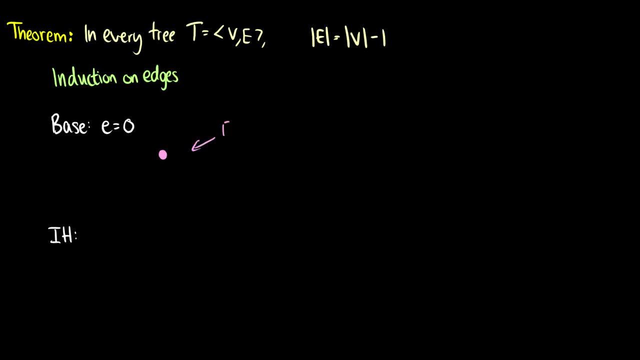 the tree, That is our tree for zero edges. Now we can see here that zero is equal to the number of vertices minus one, which is just one minus one. So the base case holds For induction. we're going to assume that e is going to be. 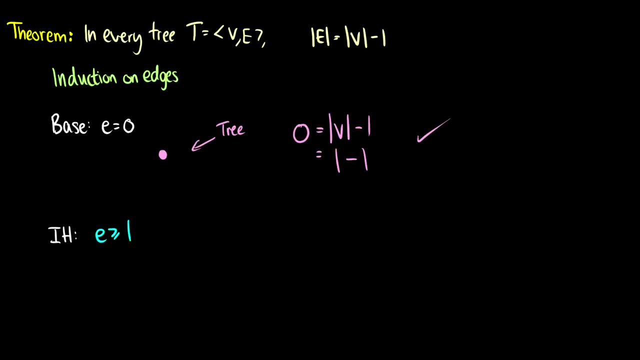 greater than or equal to one. Of course I use this little e to denote the number of edges. So we're saying that there's at least one edge here, So we know that there's at least one vertex. so we can say there's at least one vertex V in our 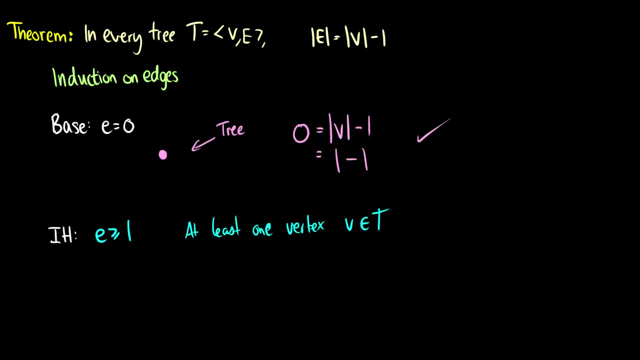 tree. so what we'll do is we'll define this new tree, we'll call this T- prime should get rid of that stick there- and it's going to be the graph T minus some vertex that we pick. so let's say before that we had a tree like this. well, what? 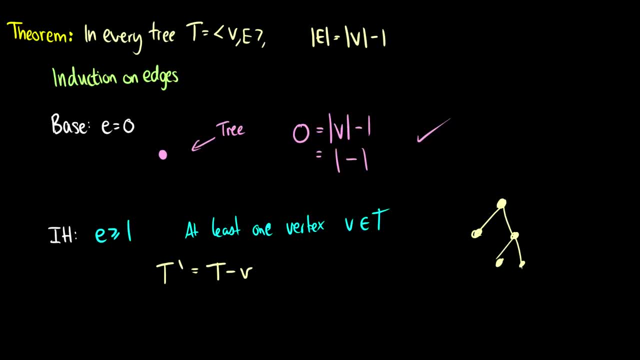 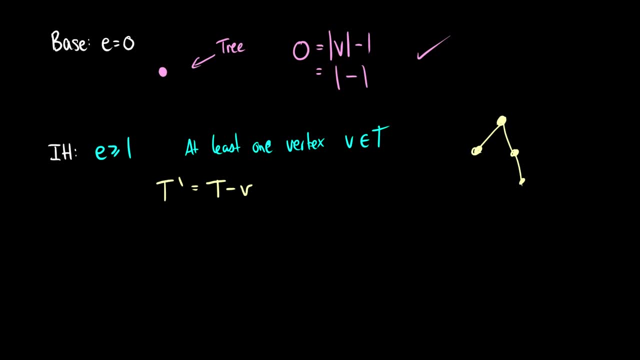 we're doing now is we're saying, okay, let's just remove this vertex here, so we have this. okay, so now we have a smaller tree. and what do we know about this smaller tree? we know that the edges in this tree are going to be equal to the. 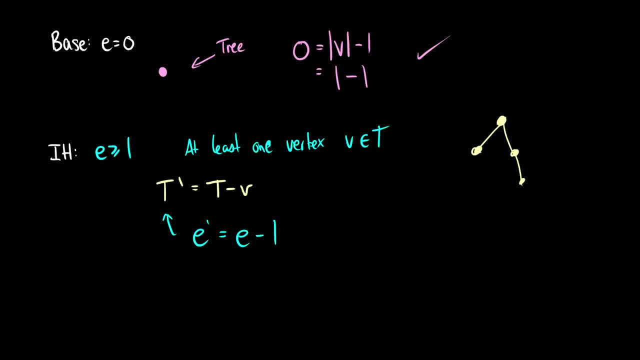 edges in the original tree minus one, because we removed one vertex, so one edge is going to come with it and the number of vertices is going to be, well, the number of vertices in the original tree minus one. okay, so what does this mean? well, if we take E prime now, we get 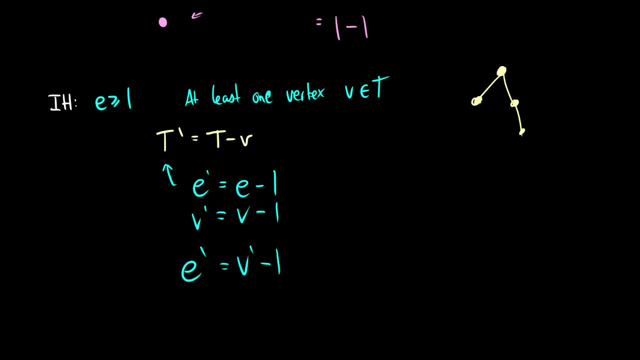 V prime minus one, because well, the induction hypothesis says that E is equal to V minus one. so when we substitute in E prime, we get E prime plus one is equal to V prime plus one minus one. so we get E prime plus one is equal to V prime. so E prime is equal to. 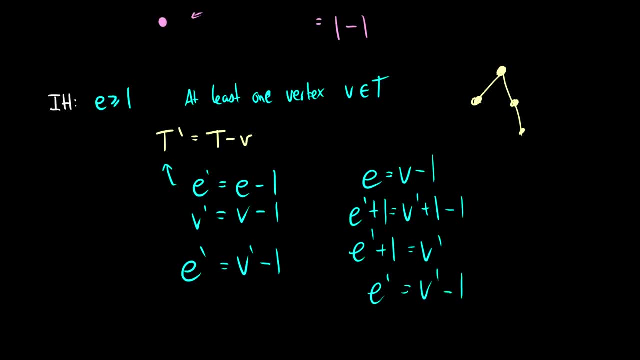 V prime minus one. so these are the steps we take at this point from the induction hypothesis. So we have proven that we have any tree with E edges, we get V minus one edges. so when we plug back in our original equation we get E is equal to V minus one. 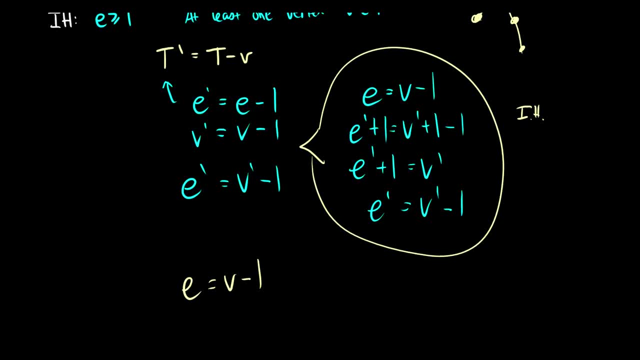 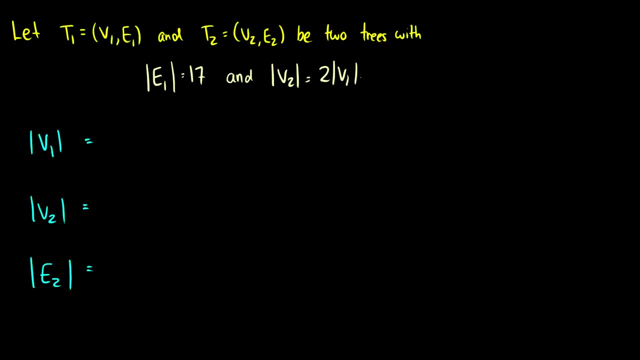 so that is a proof of the cool properties of edges and vertices in trees. So let's do a question related around this property. we have two graphs, T1 and T2, and we're given the knowledge that the number of edges in one is 17 and the 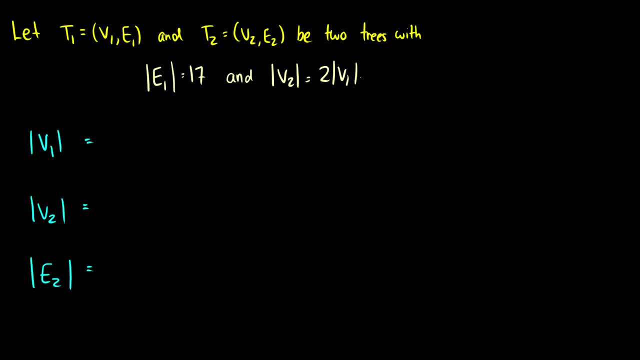 number of vertices in graph two is two times the number of vertices in graph one. So what is V1? well, remember our properties. E is equal to V minus one, so E1 is 17.. So E1 is equal to 17.. This means that V1 has to be equal to 18, because it's the number of edges plus one. 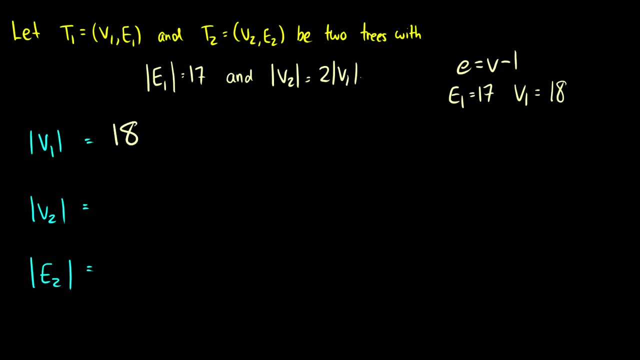 So V1 is equal to 18, V2 is 2 times V1, so that's going to be 2 times 18, which is 36, and E2 is equal to the number of vertices in graph 2 minus 1, so E2 must be 35.. 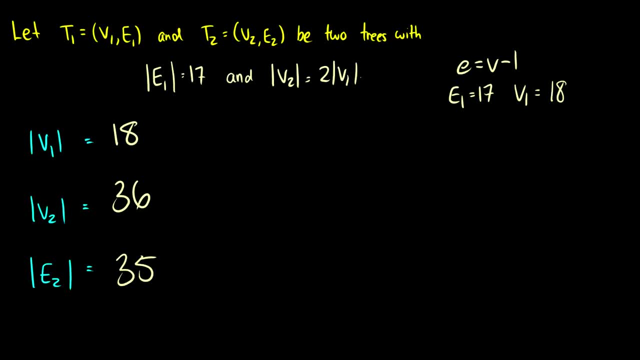 So there we go. So V2 2 times V1, 18 times 2 is 36, and of course, E2 is going to be V2 minus 1, so that's 36 minus 1, which is 35. so that's how I got that answer. that's cool. so. 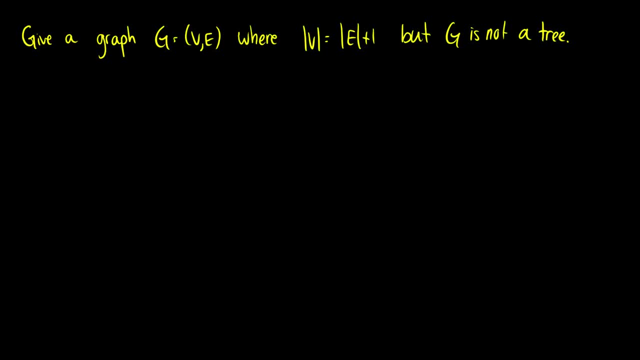 let's go to the very last thing here. is it possible to have a graph with this property, that is, the number of vertices is equal to the number of edges plus one. the same thing is saying E is equal to V minus one. I just rearrange that. 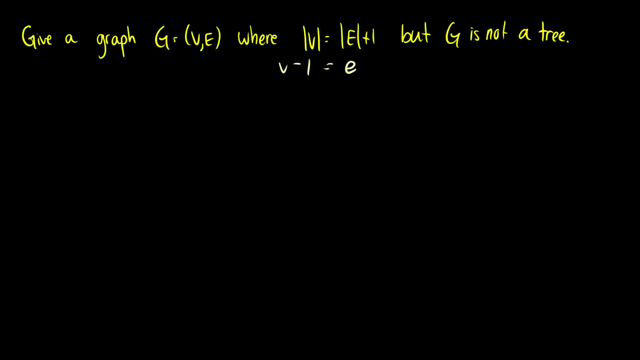 but to have this graph where G is not a tree. so is this possible? well, let's say we have three vertices, so we have three vertices, which means how many edges do we need? we need two edges, so we need to draw this so that G is not a tree. well, 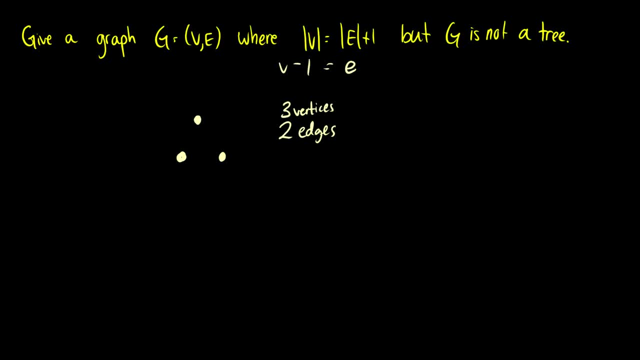 this is actually pretty straightforward, because what we could do is we could just not connect it, so that's clearly not a tree. there are other ways to do this. well, of course there are. we can do this and we can do this, so that's not going to be. 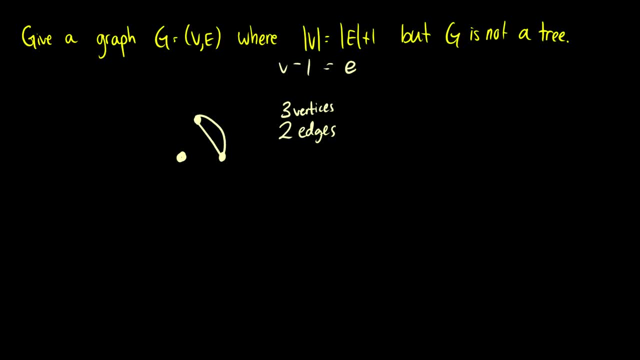 a tree. so this example is here to show you that just because we have the number of vertices is equal to the number of edges plus one, doesn't mean you're looking at a tree. you could be looking at a disconnected graph, so that's always possible, of course. if we have this, this is going to be a tree. so those are the.